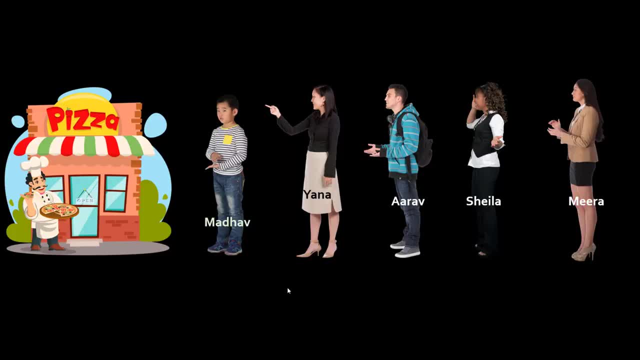 Let's say there are a couple of people waiting outside a pizza store for their pizza delivery. Now the owner of the store, Roberto, realizes that people are getting bored standing in the queue, So he offers garlic bread to each of them as a compliment. 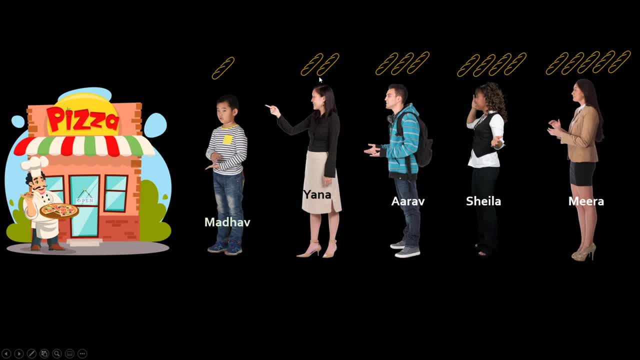 The first person in the queue gets one garlic bread. Second person gets two garlic bread. I don't know why Roberto came up with this rule, but maybe he thought that person standing in the end will be more bored, So maybe give them more reward. Now his chefs are working very hard, but still there is a delay. 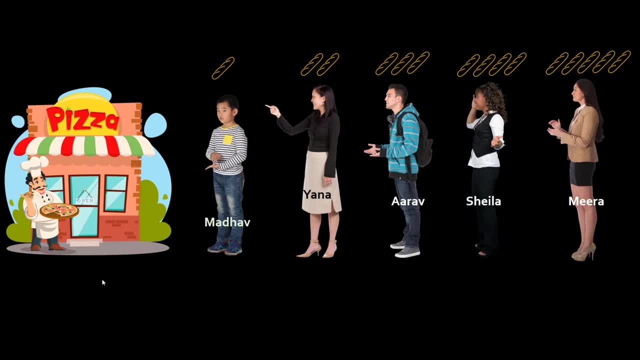 So Roberto offers one more discount, saying that you know, let me ask these people to Do some activity or some puzzle so that they don't get bored waiting in a queue. So he will say, OK, every person in the queue needs to count total number of breads that are in front of them, including their own breads. 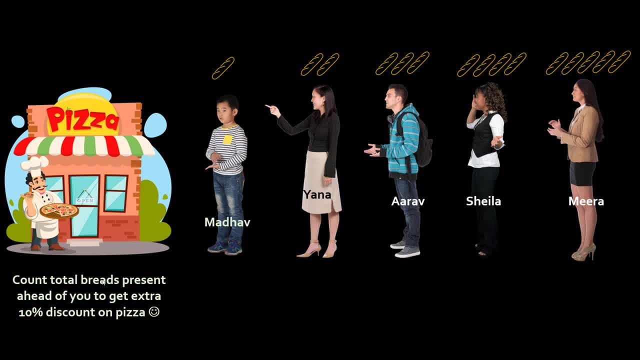 Once you give that answer, you will get 10 percent discount. So for example, for Aro it will be six, because he has three breads. There are two. So three and two five and one six. It's a simple math, basically simple. 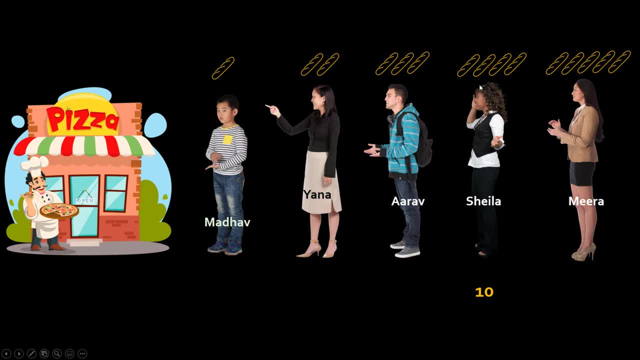 sum of all the braids which are prior to you. so for shayla it will be four and three, seven and two, nine and one ten. so four, three, two, one. you just do a simple sum. so then these people can do this sum and earn 10 discount. now, mira is actually very smart. she's smart as well as lazy. 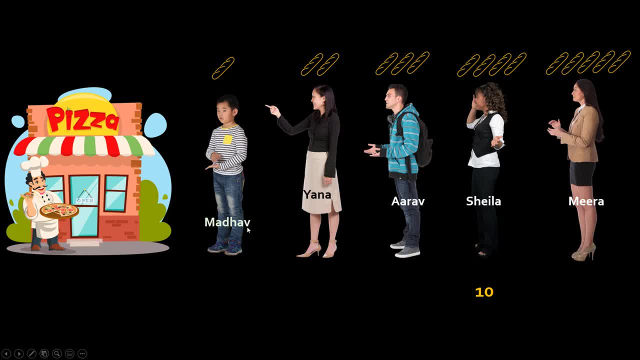 she's like: who's gonna do all the sum? you know, five, four, three, who's gonna do all of that? so let me ask shayla for her answer. so mira will ask shayla for her her answer and then she can add her braids into that and that will do the trick, correct? she can say five plus shayla's. 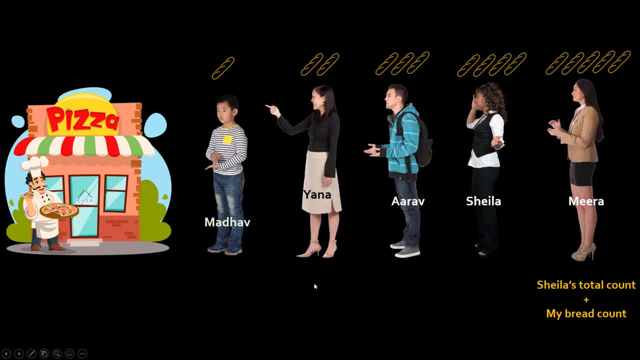 answer, which is a sum of all these answers. that will be her final answer. so then she goes: hey, shayla, what is your answer? then shayla realizes: oh, that's a nice trick, let me do it. shayla will do that trick as well. so she will ask: arau, hey, arau, buddy, what's your answer? and same thing. 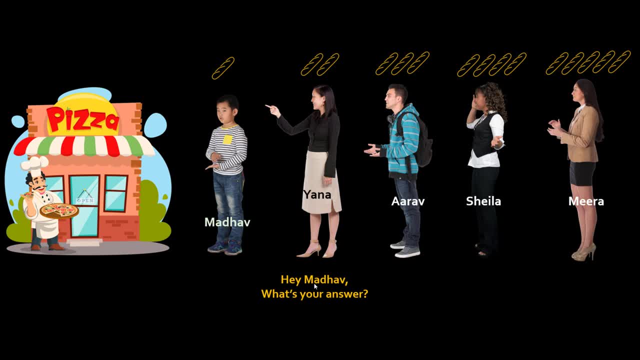 everyone will repeat until yana and she'll be like: hey, mada, what is your answer now? for mada? it's pretty straightforward. he has one braid, so mada's answer is one braid. now yana can take the answer and then she can add her braids into it. so one plus two is three. then arau can take yana's. 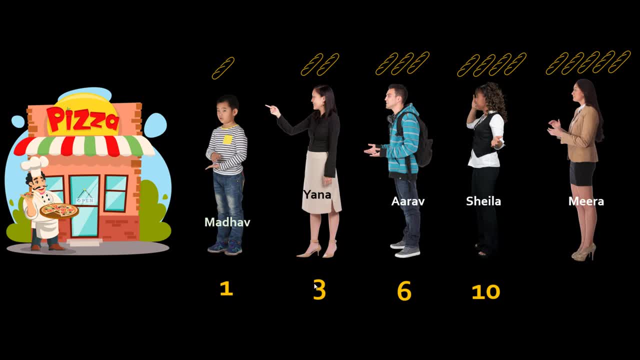 answer: add his braids three plus three, seven and eight and nine and ten and nine and ten and nine and ten and ten and nine and Six, simple math, guys and girls. Me I can say 10 and plus my five brides 15.. 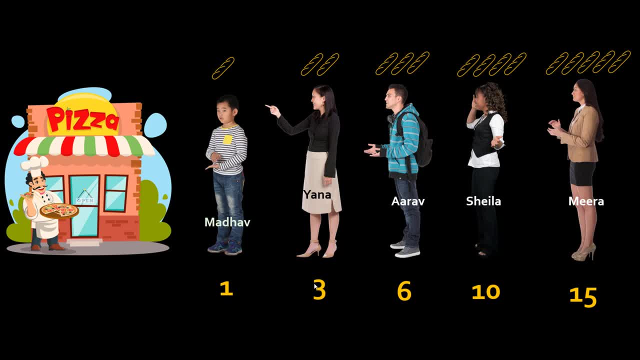 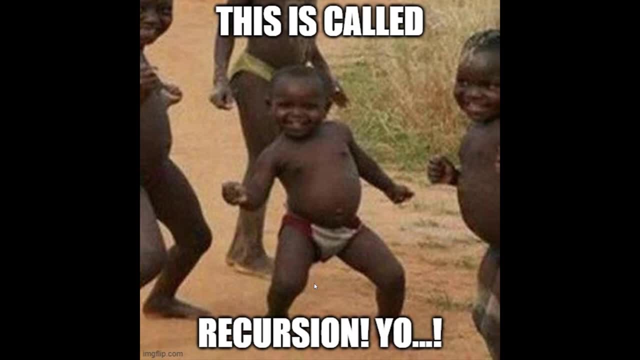 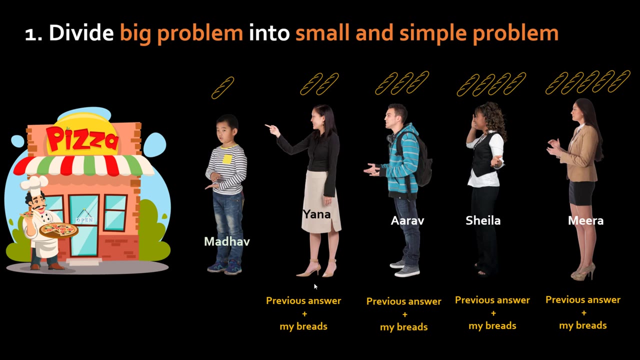 So this approach of solving a problem is called recursion. Yo, you got it. It's a very important concept in computer science. You are basically doing three steps in this approach. In the first step, you divided a bigger problem into smaller and simpler problem. 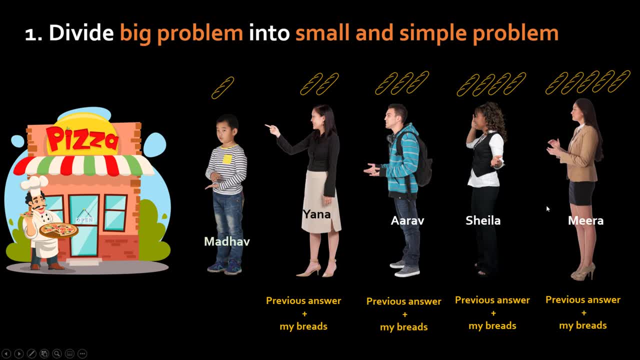 For Meera, the problem is simpler, because all she has to do is take ready-made answer from Shaila and add five brides into it, Same way as Shaila take ready-made answer from Arav, add four brides to it, and so on. 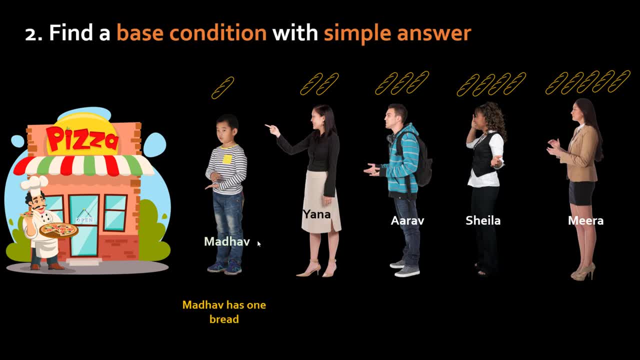 The criteria. number two for recursion is the base condition. So here Madhav's answer is one, because Madhav doesn't have any any any word in in front of him, So he can just give his answer in a second. 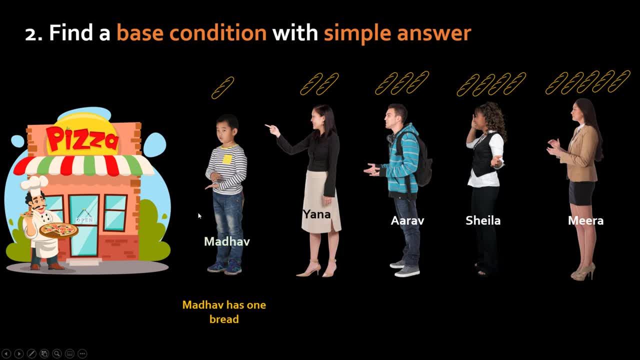 He's like: okay, my answer is one, So that's the base condition with a simple answer. So in recursion you need, you need to have that base condition. And the third point here is: once you have the answer with base condition, you roll. 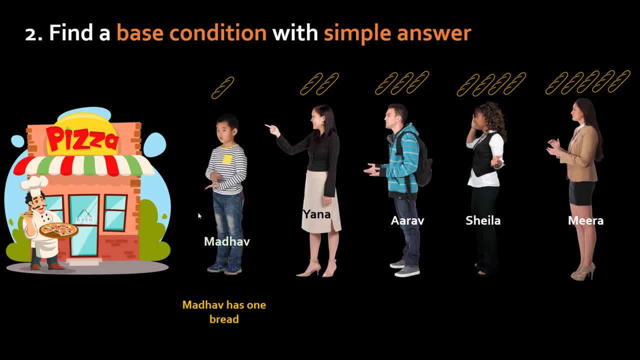 back that answer to all the way up in the chain. So now Jana will take Madhav's answer, which is one. she will add her two brides, That is three. Arav will add take Jana's answer, which is three, add his brides three, six and so on all the way. 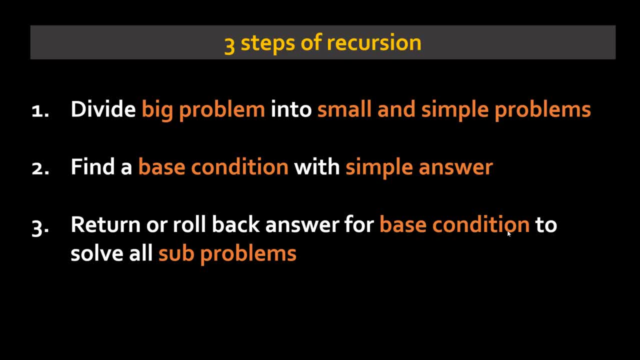 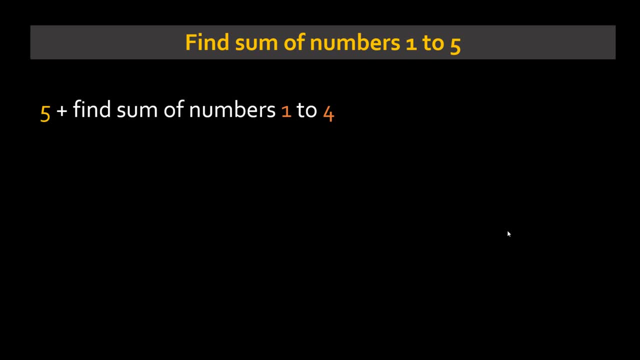 till Mira finds her solution. So just to summarize, there are three steps into recursion. So here we solve a very basic math problem which is summing up all number from one to N. Here N was five. So to sum that up, you could have used iterative approach, which is one plus two plus three plus 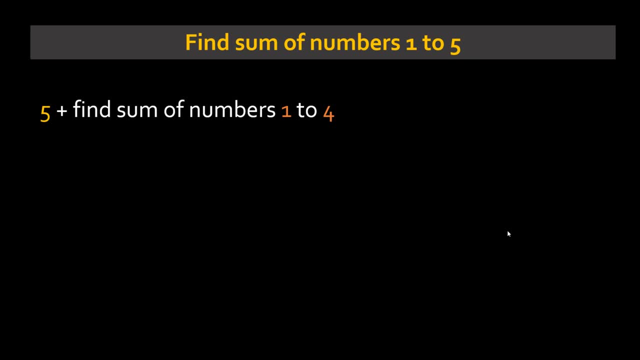 four plus five. But you have to do A lot of computation. instead. here You say five plus find the sum of all numbers between one to four. Then the second step is okay, Four plus find sum of numbers between one to three, until you find a base condition, which is find a sum of numbers from one to one. 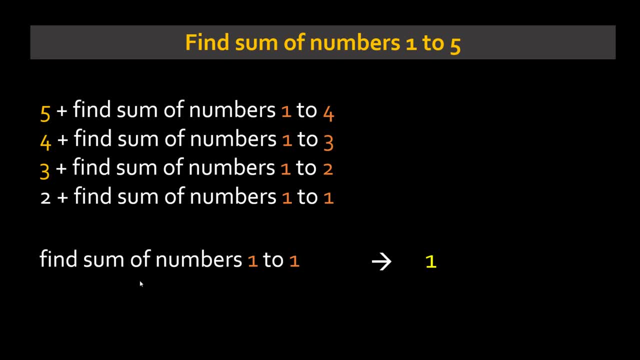 And that's pretty straightforward. It is one, obviously, And once you have the answer, you roll back. Now, see here, look at this line carefully. Okay, Fine, Some of Numbers One to one. What is it? 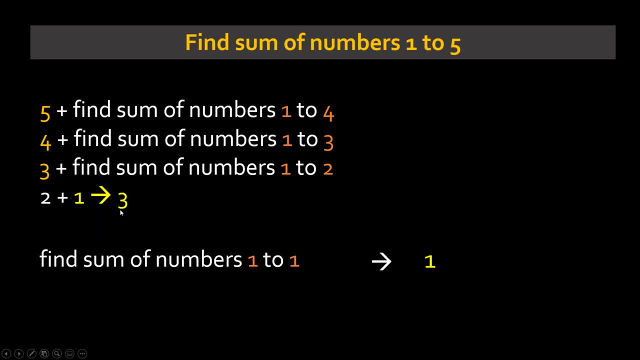 Well, it is one. Subtitute that three. All right, Three is my answer. Now find the sum of numbers one to two. What is it? Well, it is this three. So substitute this three here at top, You get six. 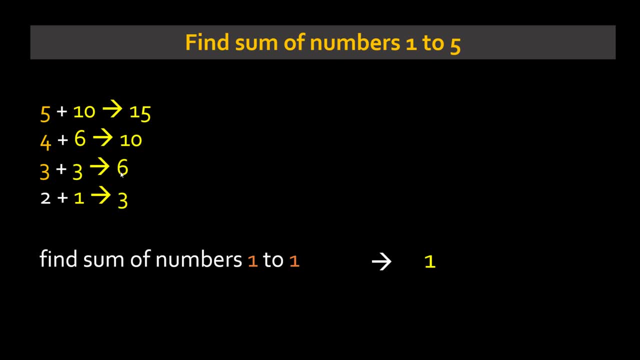 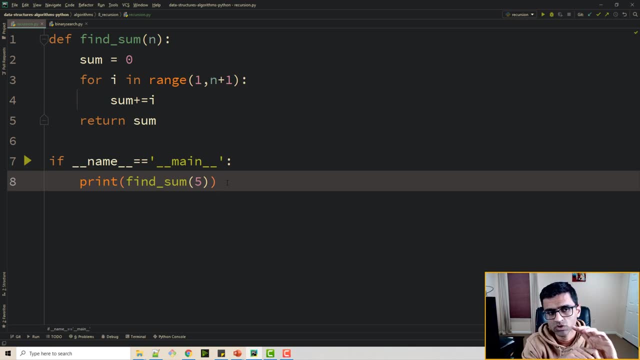 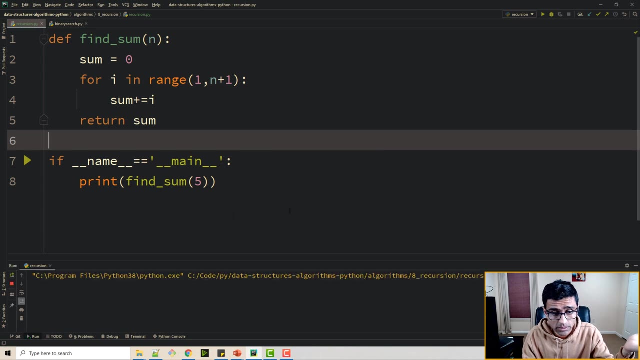 You keep on doing that till you get 15.. Now let's write Python code for same. I have opened my PyCharm community edition and I have this basic program that finds you the sum of all numbers from one to n. So for five- we already saw in the presentation- the sum will be 15.. 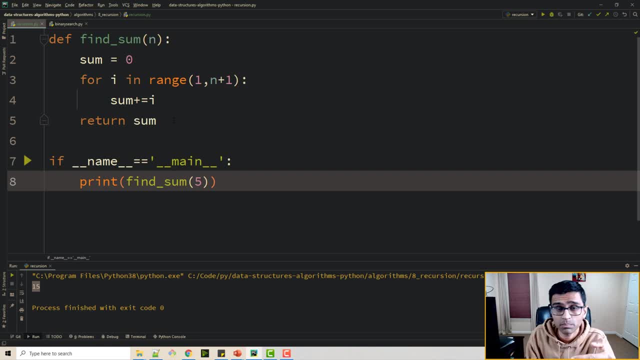 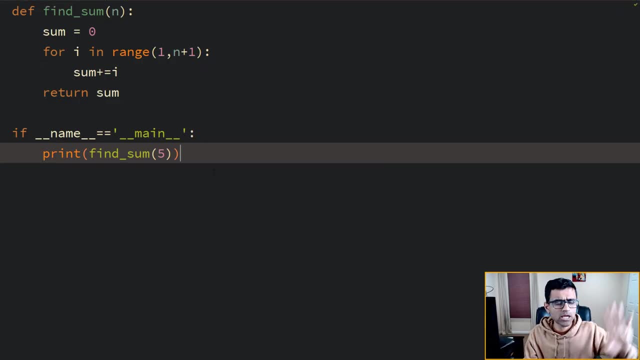 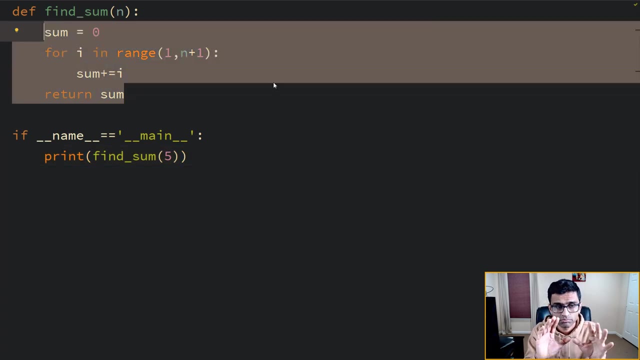 Okay, But this function is using iterative approach. It is not using a recursion. So what I'm going to do is first I will go into my meditation mode and then I will write this same function using a recursion. Okay, So, just to summarize, this function can be written in two ways. 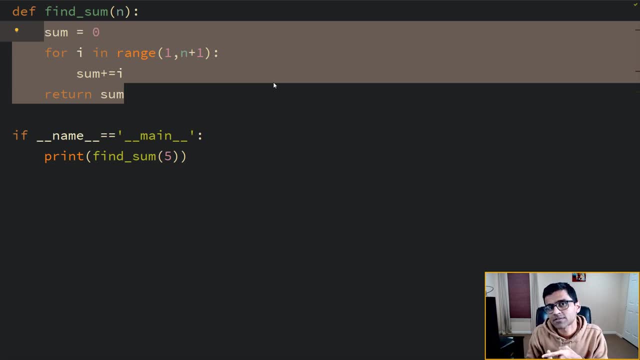 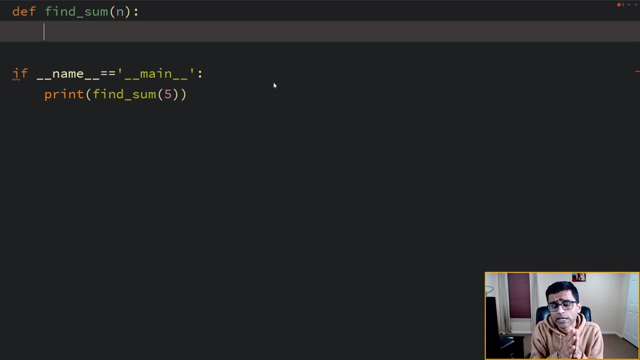 One is iterative approach, which is what you see on the screen. Second is recursive approach. Okay, So now let's write that function. What we saw in recursive function was two criterias. One is the repetitive task that you are doing and you are reducing the problem to smaller and smaller problem. 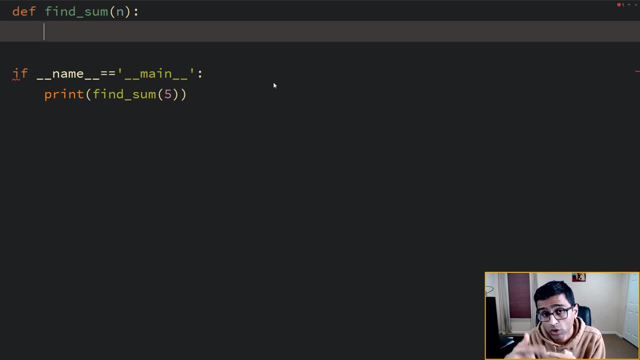 And the second one is the base condition which will terminate your recursion. So let's tackle the recursive criteria first. So sum of n number is nothing but n plus. find sum of n minus one, Right. So we saw Mira, like her braid count. is her braids, which is her answer. is her braids, which is n. 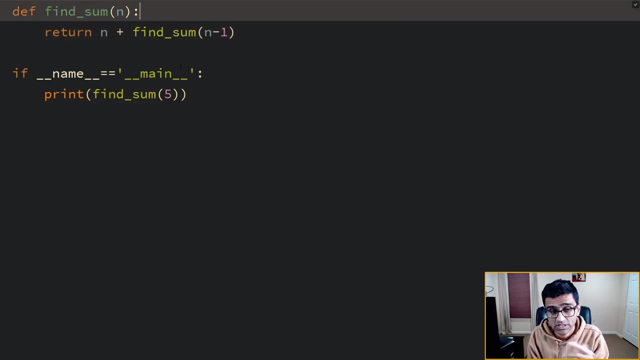 And then the answer that Sheila had. you know previously. So that is this condition. Now, if you just run, the score is going to, of course, go into infinite loop because you're not terminating. So you need base condition to terminate. 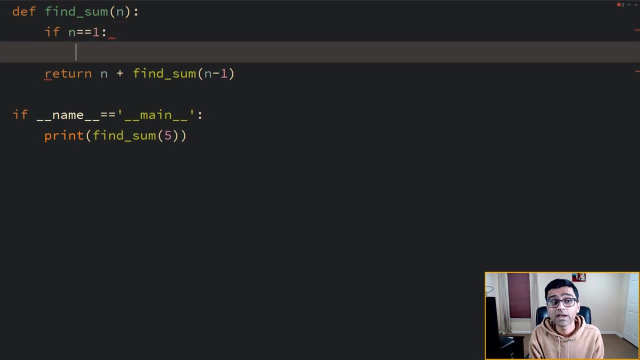 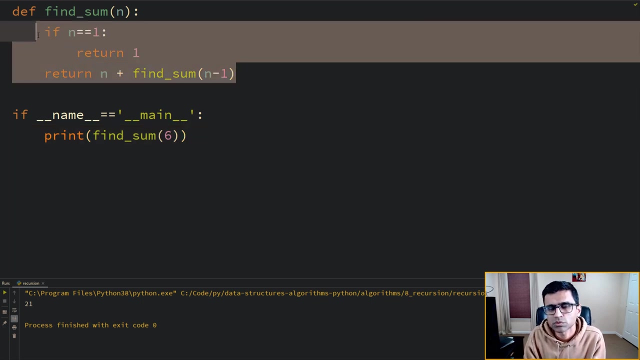 Now, what is base condition? Well, one One. if n is equal to one, then you return one. Okay, So now let's run this code. See it executed it? fine, If you say six. Now the beauty about this code is it is so simple and very intuitive to read. 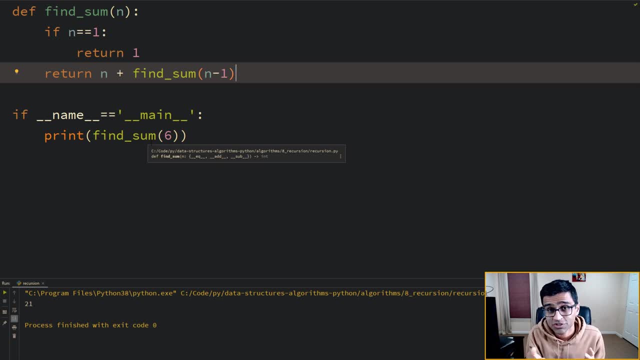 Is this: that you have to be a little careful about infinite conditions when you are writing recursive code. Right, That's one of the things we can do Often if you're stuck in some problem of what helps is debugging, So let me just debug this code. 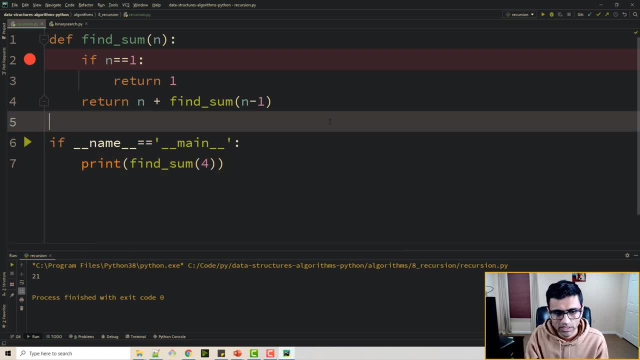 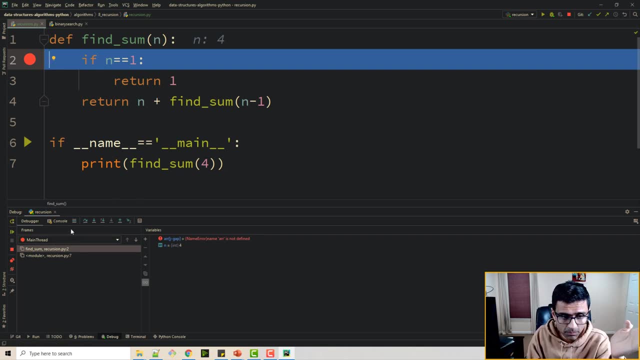 Okay. So I will do it for, let's say, four Okay, And if I run right click debug it will show you the first call for n equal to four. Okay, Now watch this area. this area, the stack will grow. 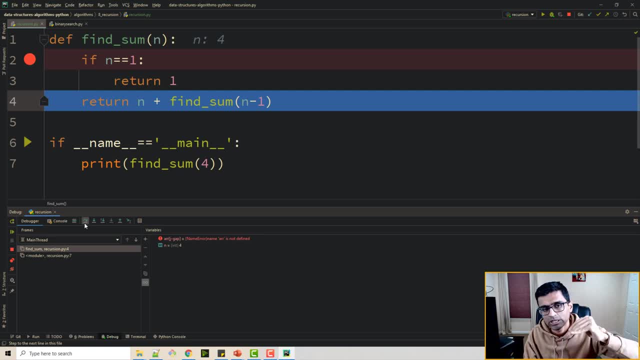 So if you do f 10, what will happen is now it will call: find some function for n equal to two. Okay, So you have this in f 10.. Right, Okay, Got it. We will see. now it shows a bunch of more characters. 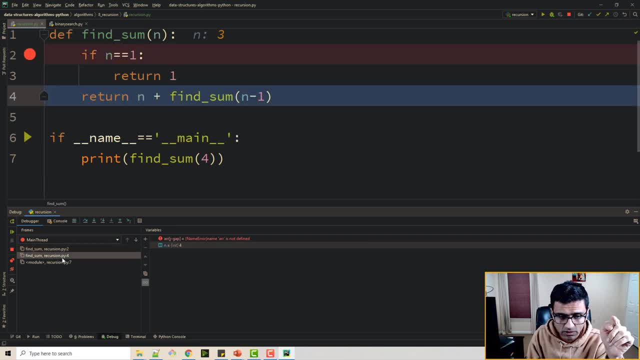 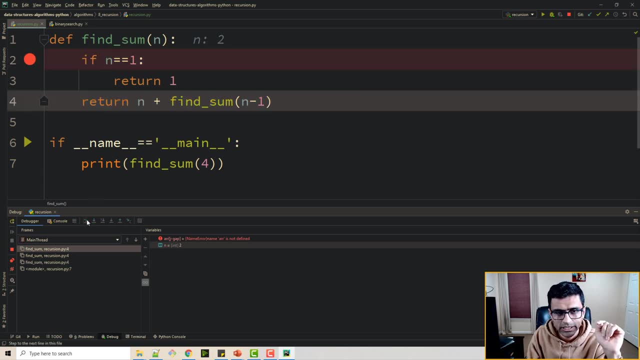 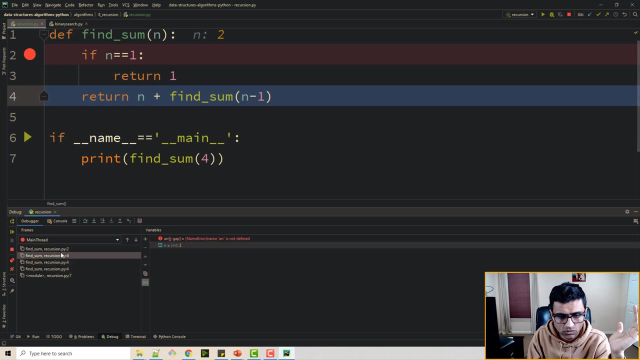 three. you see n equal to three and you see two calls now here. the first call was n equal to four. second call is n equal to three. when you go deep down, it will keep on calling it see, i have now four calls in my stack: n equal to four, three, two, one. now when i hit one, i'm hitting a base condition. 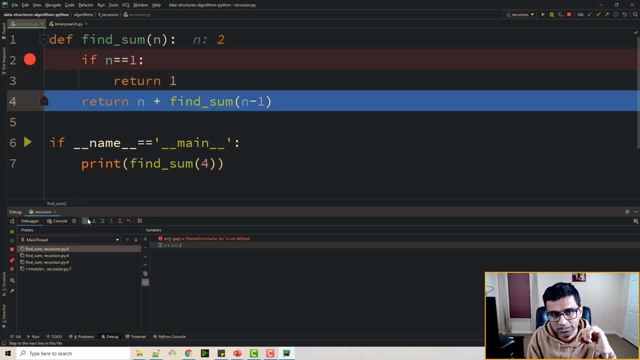 and it will return from here. so when it returns. now i'm unwinding my stack. this is called stack unwinding. okay, and this function would have returned value one. so now i have n equal to two, so two and one, so i'll get three. okay, then i go back again. so i'm unwinding. okay, now i'm back to 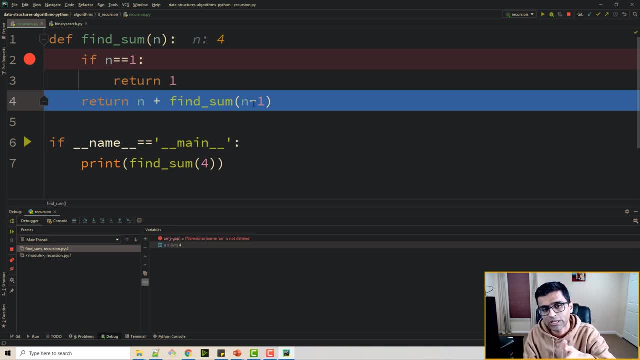 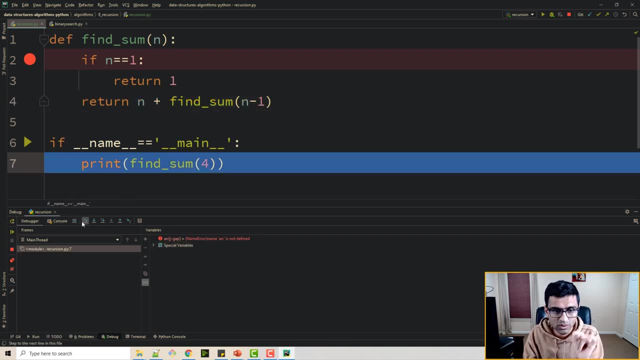 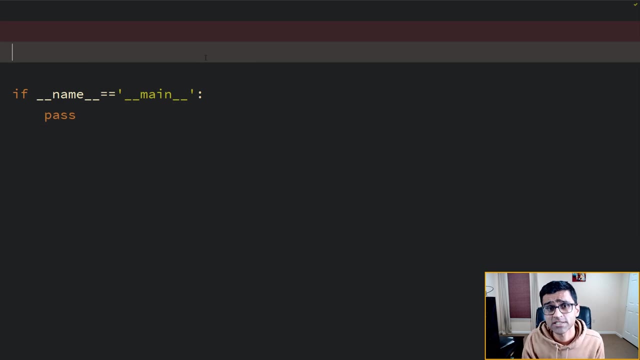 four. so back to four, so four and the find some value of three will be what? three, two, five and one, six, so six and four, ten. so now, when i go back here, ten is printed. let's look at fibonacci series problem. so fibonacci series starts with zero and one. 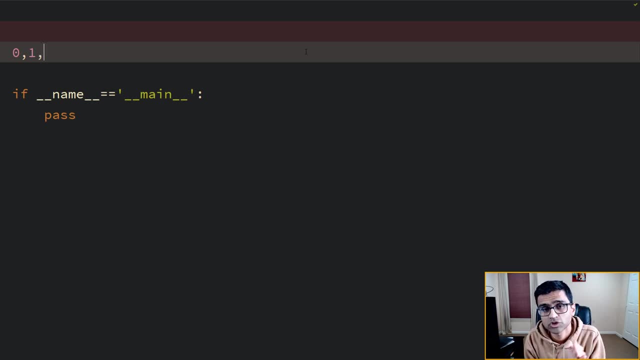 and then you generate new numbers using the sum of last two numbers. so what is the sum of zero and one, one? okay, what is sum of one and one, two, last two numbers you have to add. so two and one is three, two and three is four, two and three is five. sorry, 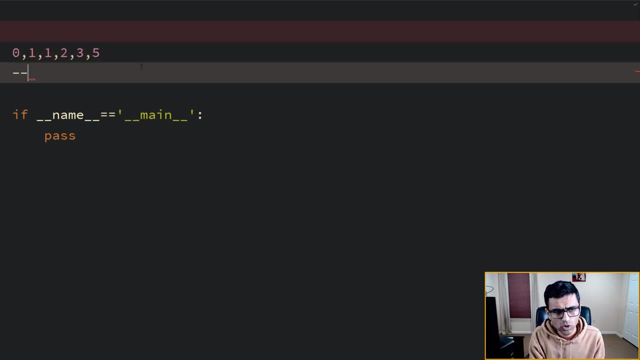 that's it, fibonacci series. and if you talk about the indexes, okay, so this is at index zero, this is one, this is like array index three, four, five, six. okay, so this will be five and three, eight. now i'm going to write a function called fib which will take n, so this is the fibonacci number at nth position. okay, so for 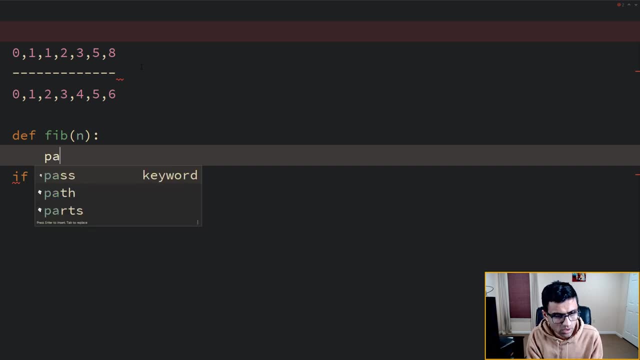 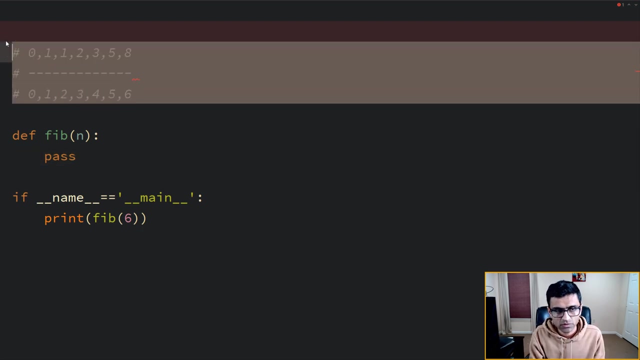 example, if i do oops, so if i do fib, so if i do fib six, for example, at position six i have number eight, so this function should return me eight. okay, so that's what we are going to do now. fibonacci series also is a recursive problem, because at every step you are repeating the same solution which is at any given position. 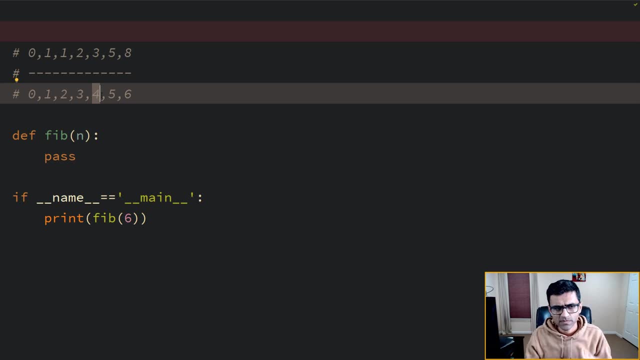 you want to find out the sum of previous two numbers. and what is my base condition? well, my base condition is: if fib of n is zero, then it is zero. if n is one, then it is one. so let's take care of that condition. so if n is zero or n is equal to one, then you want to return n. okay, so if you call this function, 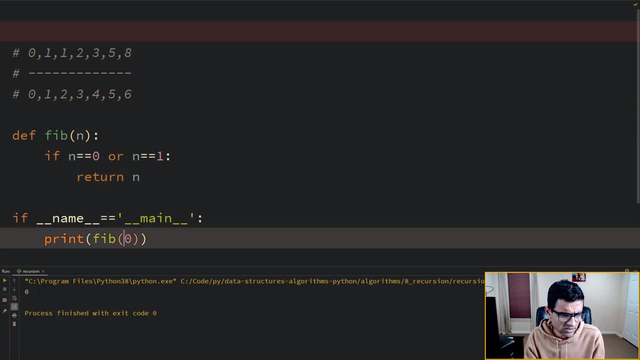 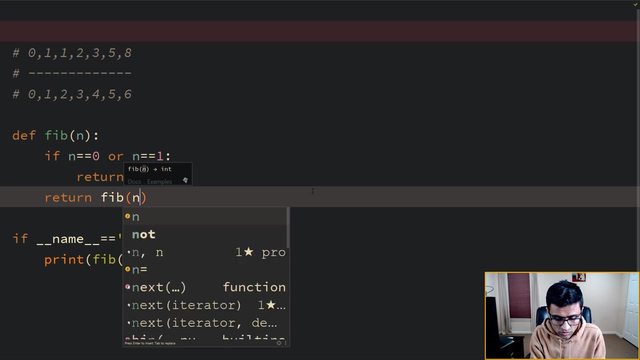 for zero and one it's going to print see it printed. zero for zero, it printed. zero for one, it will print one. so my base condition is satisfied. now let's write a recursive condition, which is fibonacci. number again is a number of previous two numbers, which means n minus one plus n minus two, and 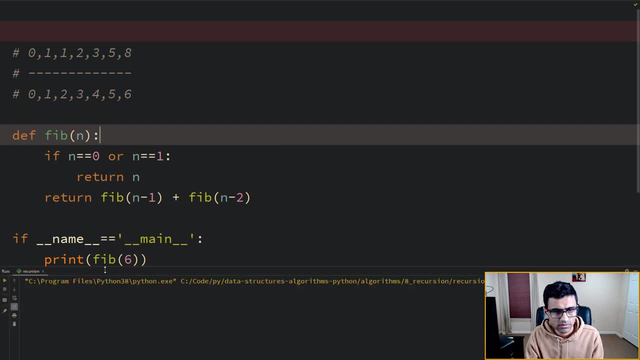 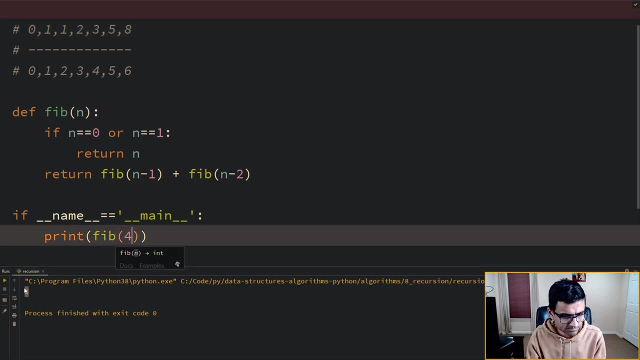 when i do six here, voila see eight. okay, if i give four i should get three, so let's give four. you can run it for any number. let's say ten number like tenth number will be like 55, okay, so you saw that the code looks so simple and very intuitive. 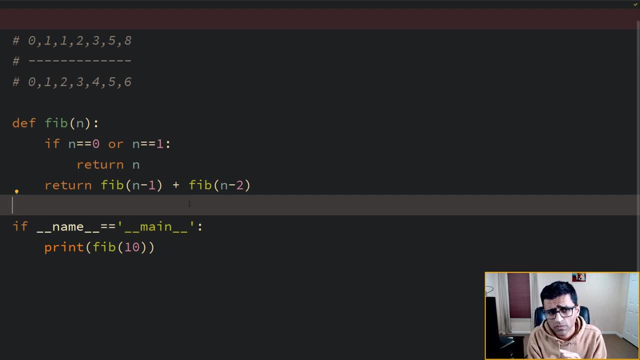 you just need to take care of infinite conditions and all that. but otherwise the code is very intuitive and in computer science interviews they generally ask recursive questions. so if you want to become a good programmer or crack computer science interview, you need to have very good understanding of 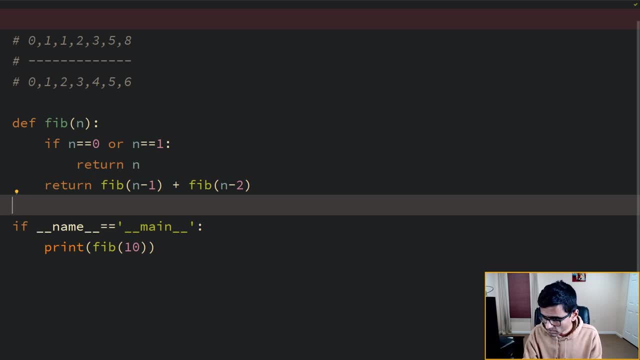 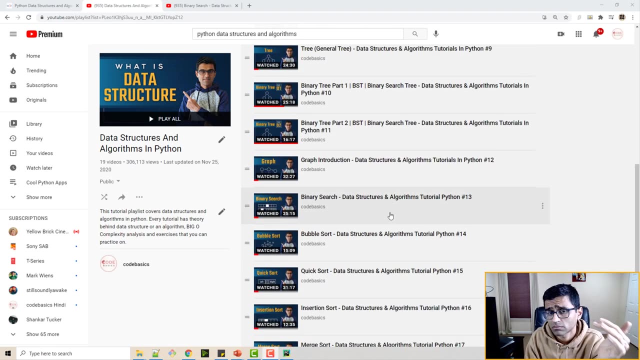 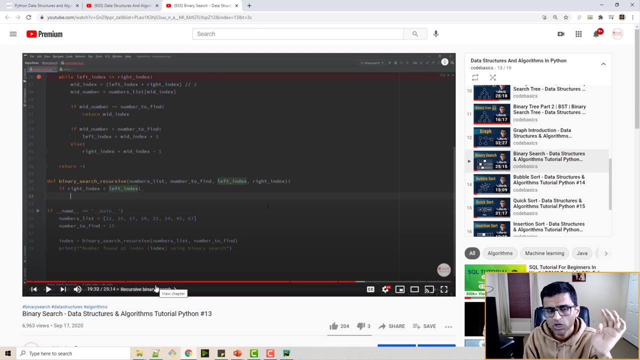 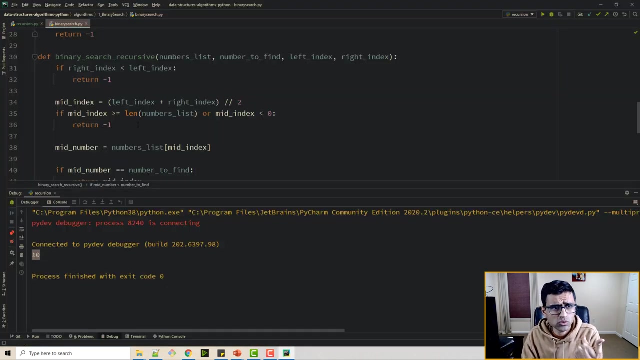 a recursion. now I have this complete Python data structure and algorithm tutorial playlist where I covered, actually, binary search. okay, and binary search can be solved using recursion. so if you watch this video properly, you will get to know how binary search can be solved using recursion. so I'm gonna quickly show you that code as well. so this is for binary search using. 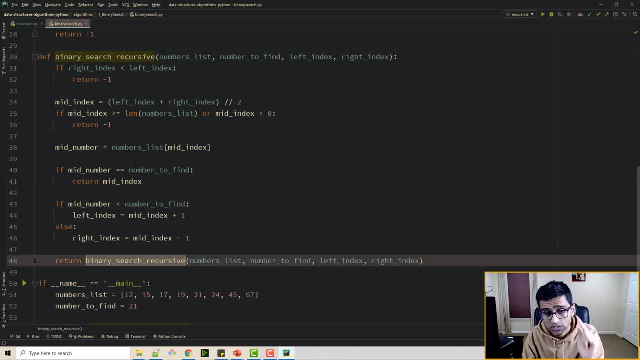 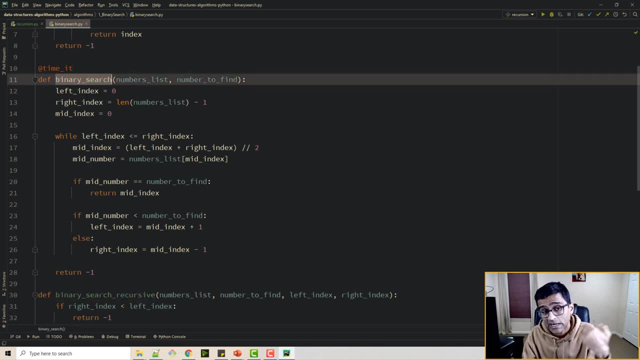 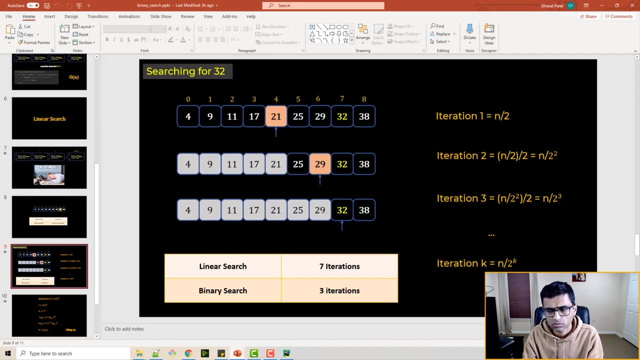 recursion. so here you see, binary search recursive. I'm calling it, I'm calling the same function within that same function. okay, binary search can be done using iterative approach as well, but recursion is a second approach that you can take. now, if you don't know about binary search, I can, I can quickly go. I mean, I will suggest you watch that video. 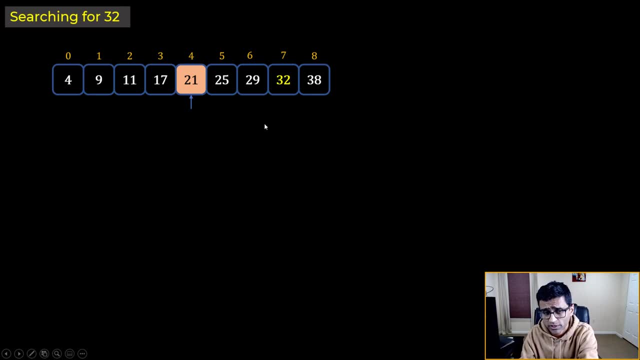 but it's simple. like you have a sorted array. this is a sorted array. you want to find any number. let's say I'm searching for 32. you start in the middle. then you say okay, 21, is it less than 32? or greater than okay, it is less than which? 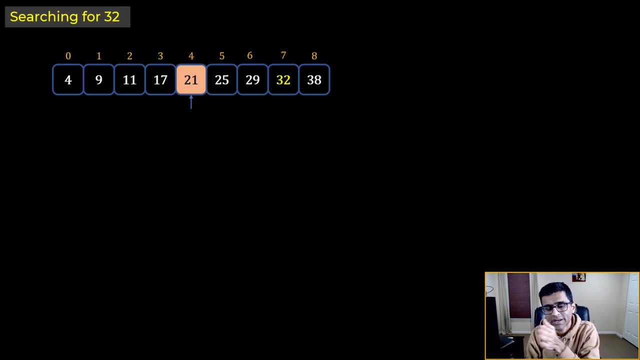 means my number 32 has to be on the right hand side, so my left hand side is ruled out. see, they are all gray. then whatever array is left on the right hand side, you again take the middle and you compare. okay, 32 is left or right? well it. 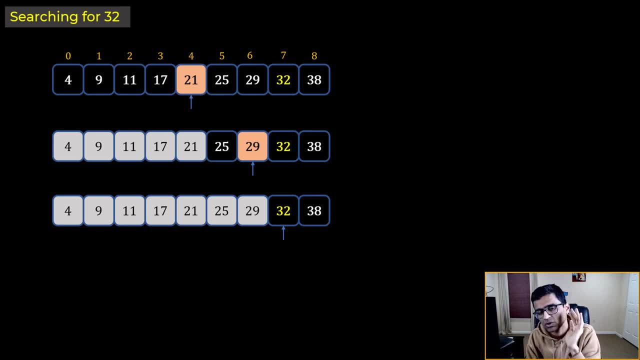 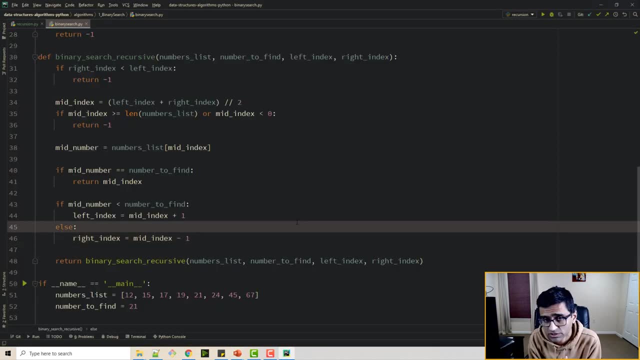 is on right, so again left hand side is ruled out. and then you find next iteration. you find this number 32 and you realize that this is also a recursive problem, and for that reason we can use the recursive methodology to solve this problem easily. now I want you to work on some exercises, so I'm going 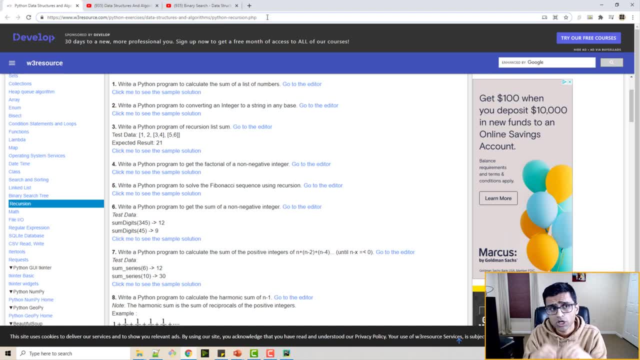 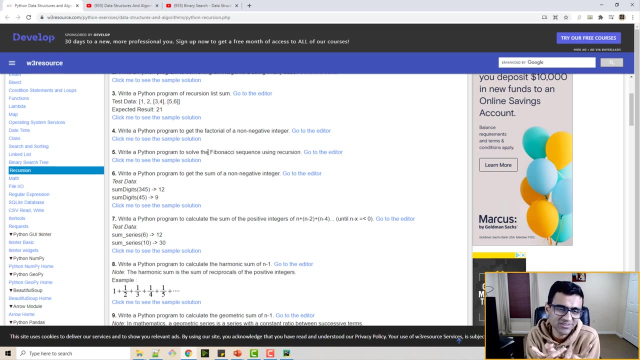 to provide a link of these exercises in video description below. w3 resources is a very good website where you can practice Python or recursive problems. so here there are various recursive problems given. here there are various recursive problems given along with the solution. but do not look at solution. you know what's going to happen if you.